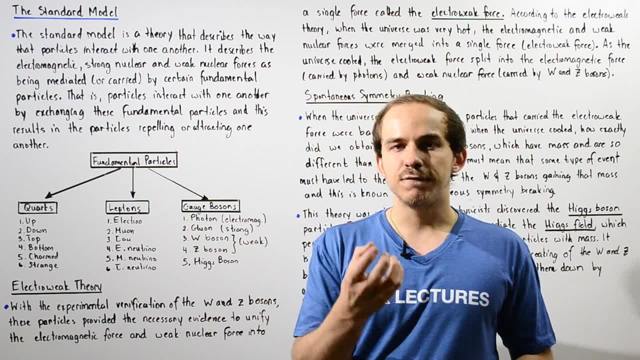 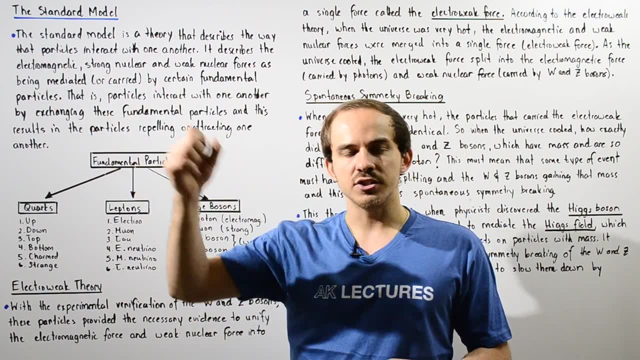 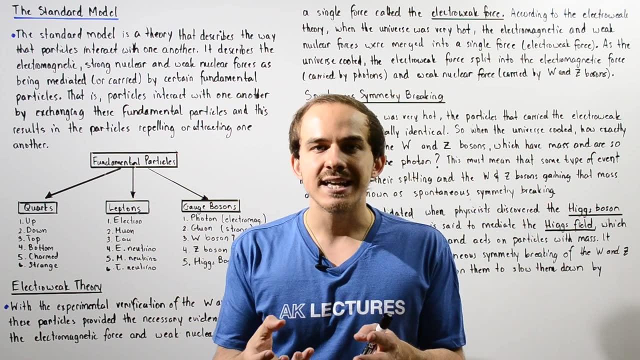 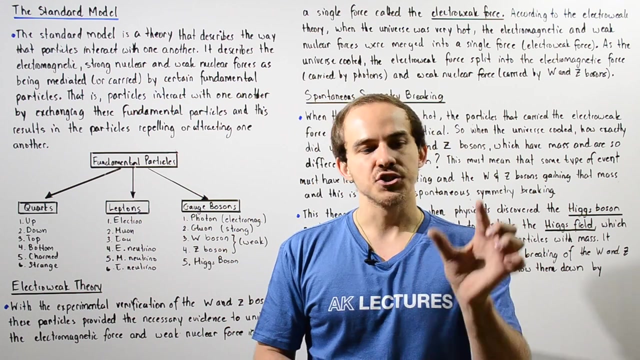 one of those electrons will release a photon And as it releases that photon, that electron recoils and travels in the other direction to conserve momentum. Now, as that photon travels, that photon is said to carry or mediate the electromagnetic force that exists between our two electrons. And when the second electron gains that photon, 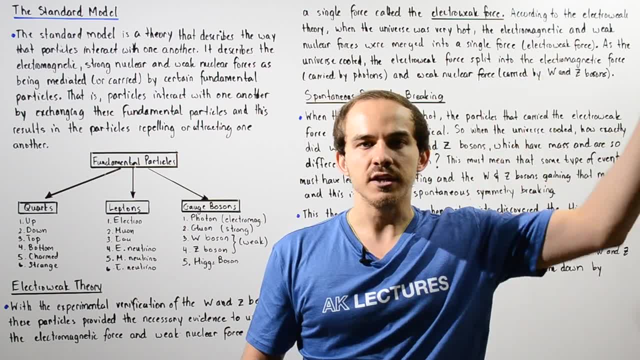 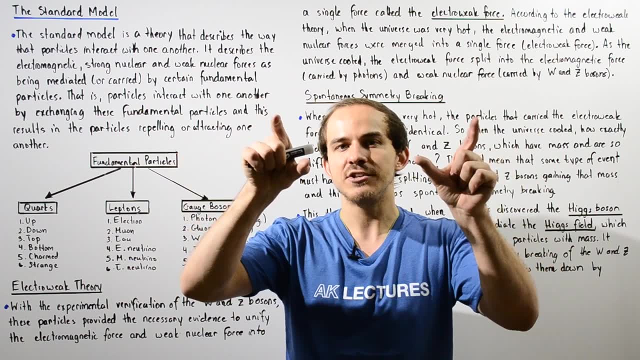 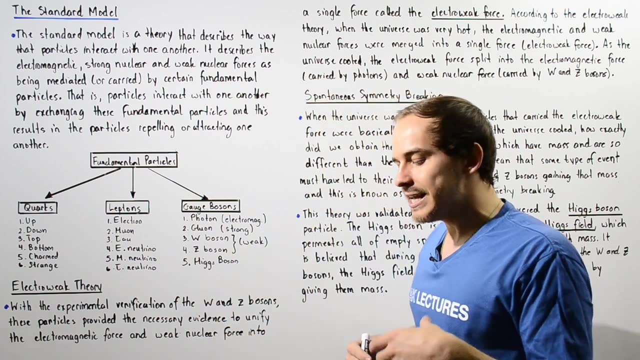 it absorbs that, That photon, and also recoils and travels in the opposite direction. So our two electrons approach, eventually they exchange that photon that carries the electromagnetic force and travel in the opposite direction. So and in this manner, particles interact with one another by exchanging. 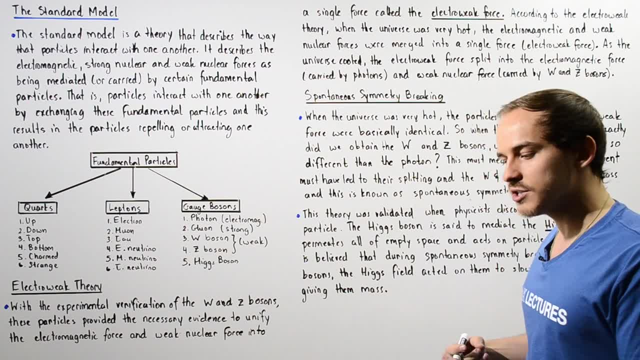 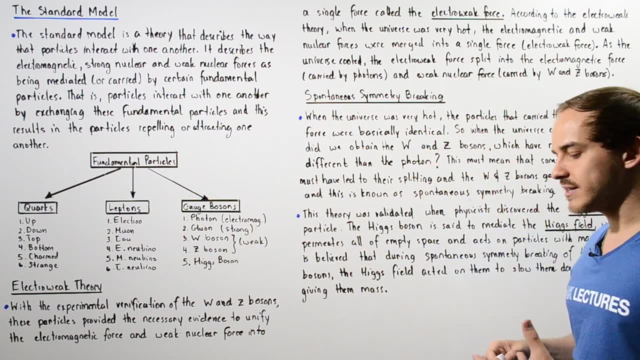 these fundamental particles that are carriers of our different types of forces, And this is what the system is capable of doing. So let's say that we have a photon that carries an electromagnetic standard model basically tells us about how the particles interact with one another. Now 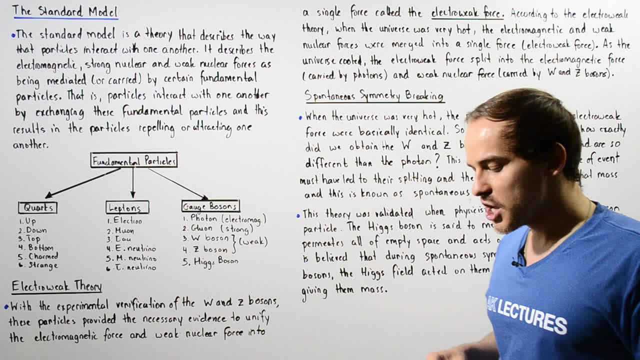 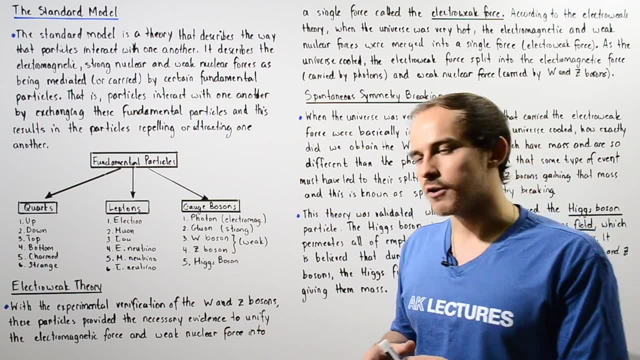 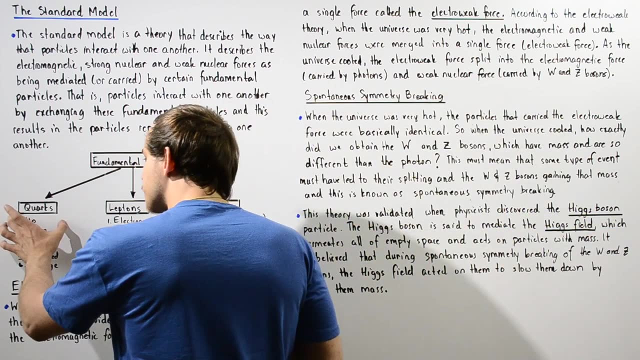 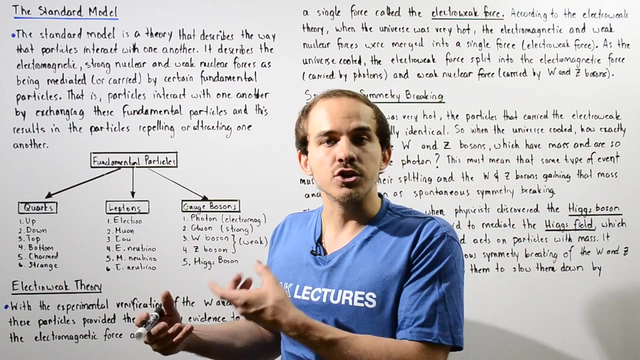 there are many different types of fundamental particles. A fundamental particle is any particle that is believed to have no internal structure, And there are three major subcategories to the fundamental particle. So we have the quarks. The quarks are basically those fundamental particles that compose other particles, known as hadrons, For example. one type of a hadron is 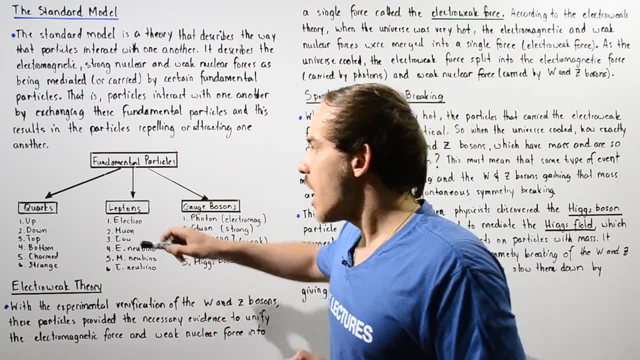 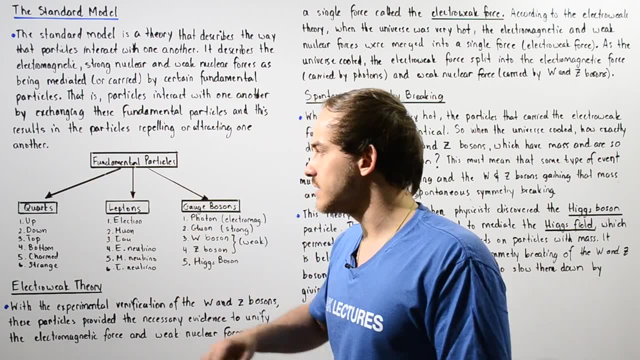 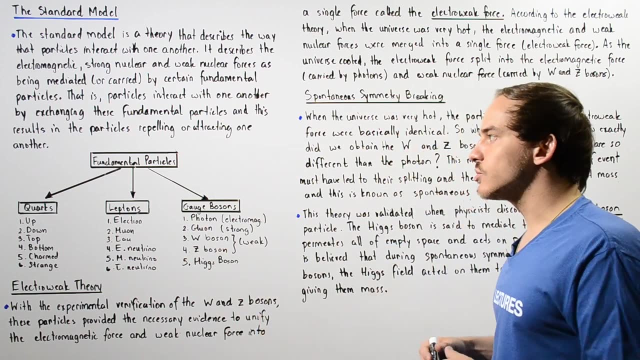 the proton, And the proton consists of two up quarks and one down quark. Another example is the neutron. The neutron consists of a single up quark and two down quarks. Now another type, another subcategory of the fundamental particle is the leptin. 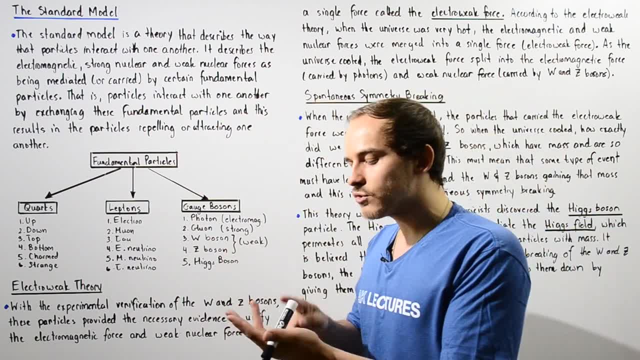 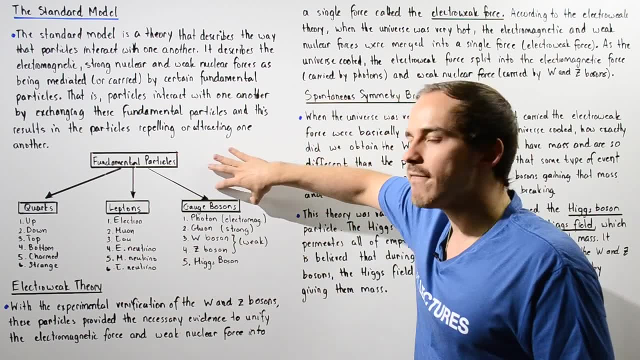 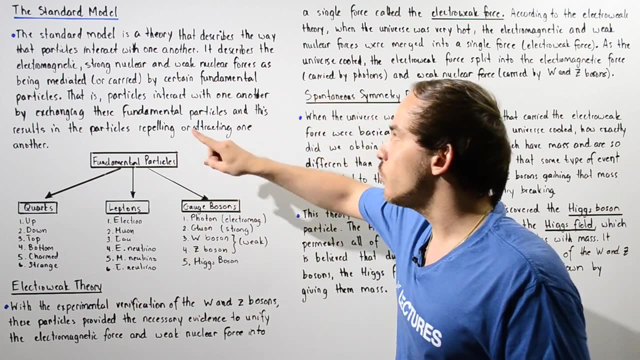 So we have six leptons, We have the electron, the tau, the muon, as well as their corresponding neutrinos, And finally we have the gauge bosons. The gauge bosons are those fundamental particles that we discussed earlier. So these are the particles that are said to carry or mediate. 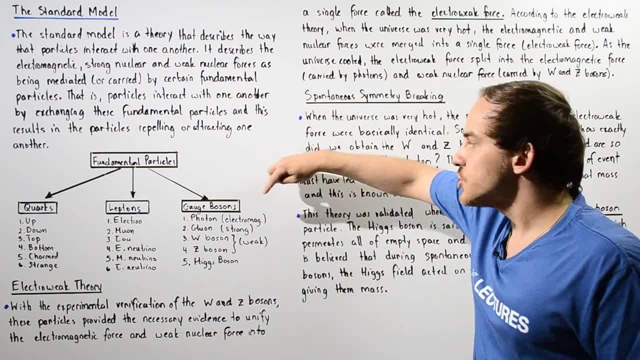 the different forces that exist in nature. So we have the photon, which carries the electron and the neutron. So we have the neutron, which carries the electron and the neutron. So we have the electron, which carries the electron and the neutron. So we have the electron, which carries 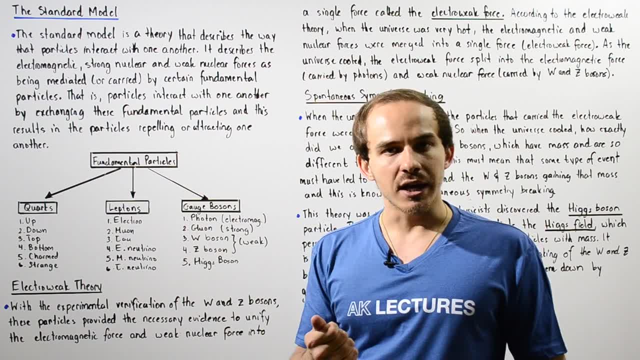 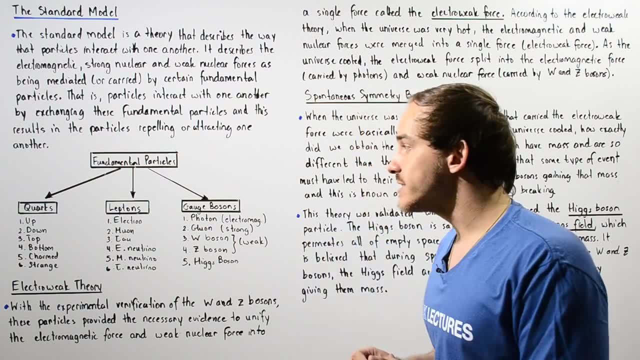 the electron and the neutron. So we have the electron, which carries the electron and the neutron, As we described earlier. we have the gluon, which is said to carry the strong nuclear force, also known as the color force, For example, the way that the quarks combine to form the proton. 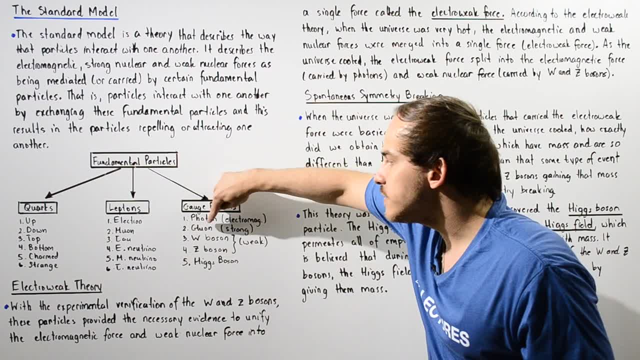 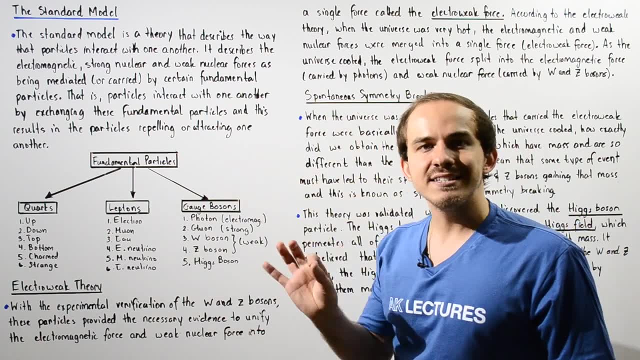 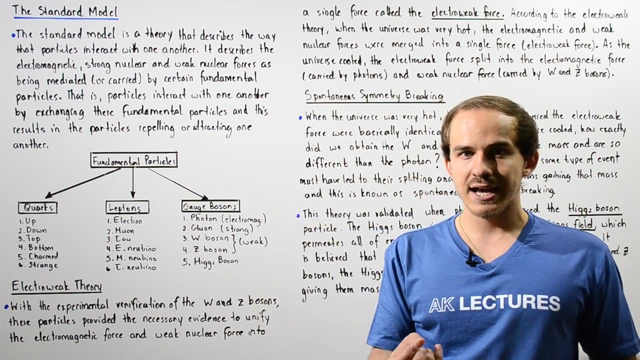 or neutron is by exchanging these fundamental gauge bosons known as gluons. So next up we have the W and Z bosons. These bosons, these particles, are the leptin, And the leptin is said to carry or mediate the weak nuclear force. So basically, if we examine radioactive decay, 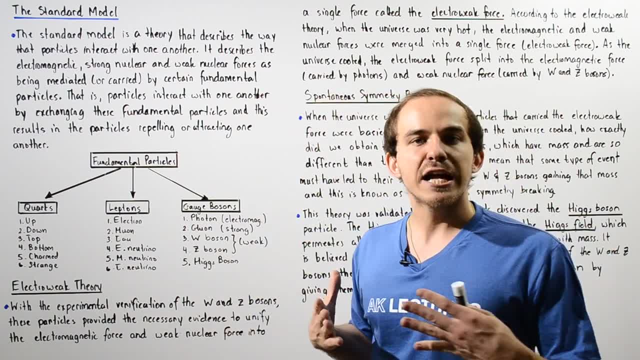 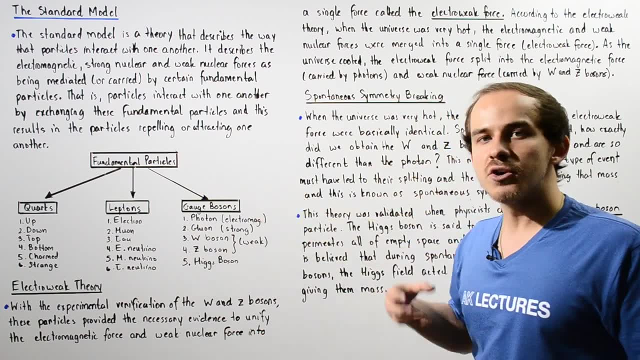 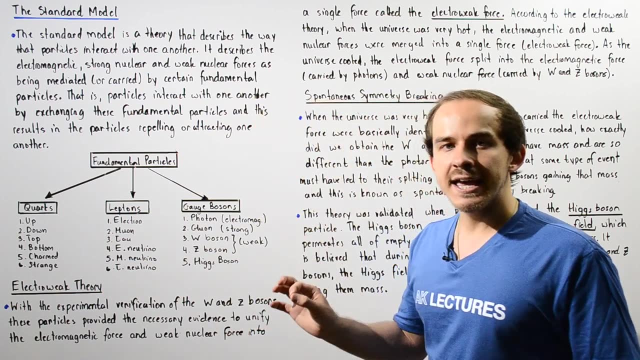 for example, the beta-negative decay. that beta-negative decay takes place as a result of these particles that carry the weak interactions, the weak nuclear forces, And finally we have something known as the Higgs boson. The Higgs boson is said to carry the 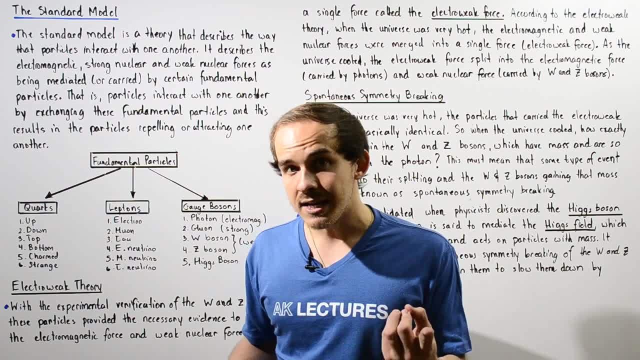 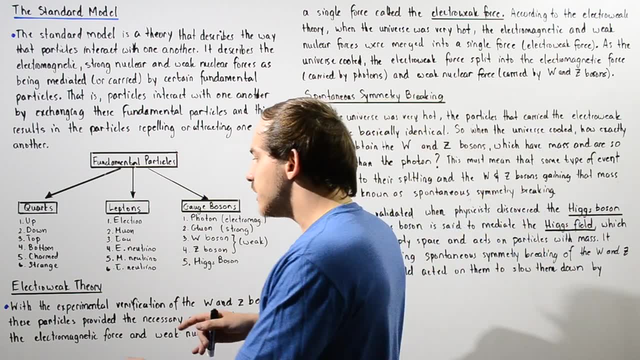 weak nuclear force. So what is the Higgs boson? Well, the Higgs boson is a particle that is said to carry or mediate our Higgs field. that we'll talk about in just a moment. So let's move on to the electroweak theory. So what exactly is the electroweak theory? Well, 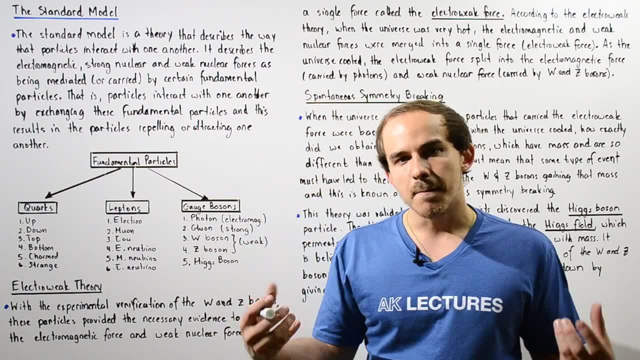 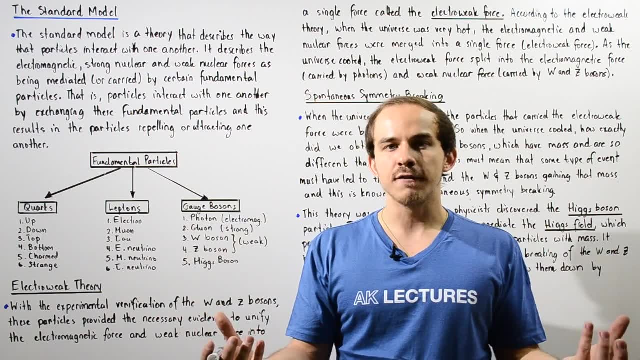 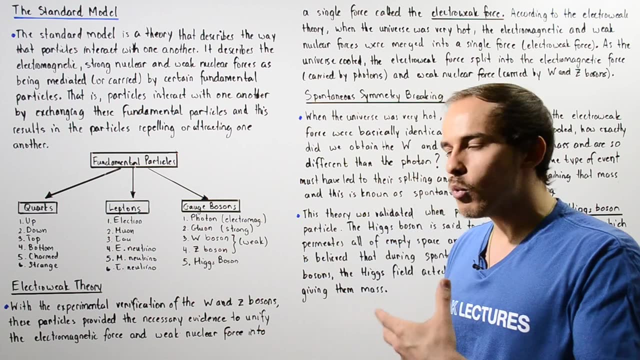 the electroweak theory is a theory that basically combines or unifies the two different forces, the electromagnetic force and the weak nuclear force, into a single force of the particular force known as the electroweak force. So basically, with the discovery of the WNZ boson, the discovery and 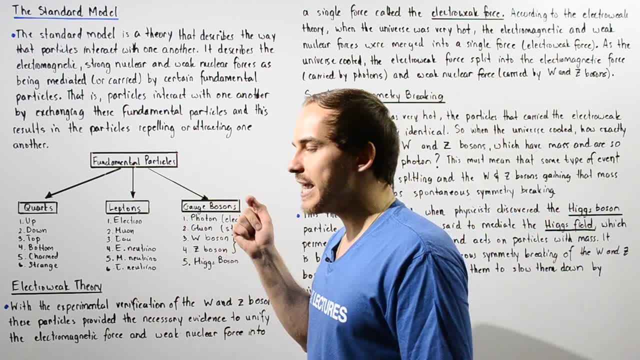 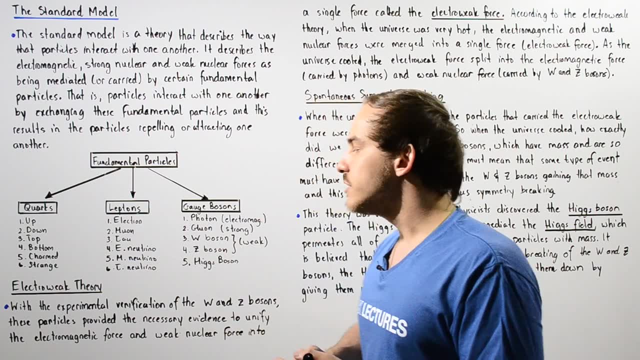 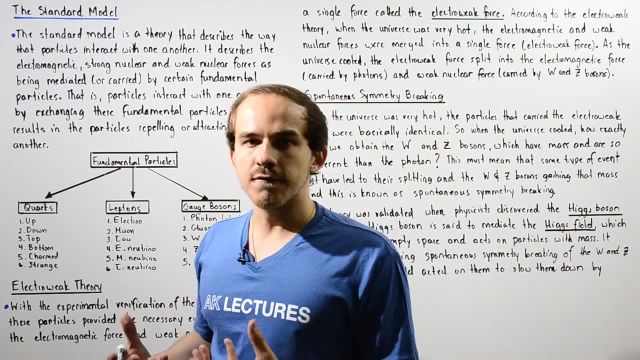 experimental verification of these two gauge bosons led to the validation of the electroweak theory, as did the discovery of the Higgs boson, as we'll see in just a moment. So basically, when the universe was very, very hot. what this theory states is the following: The photon. 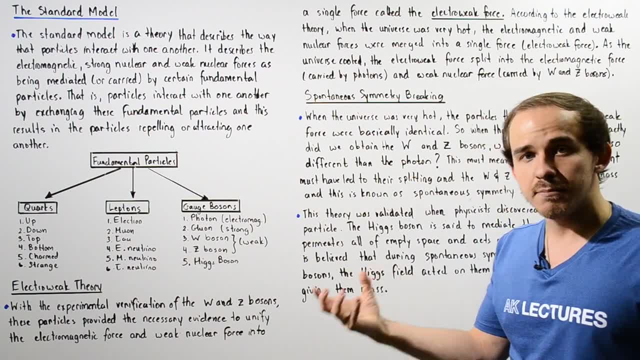 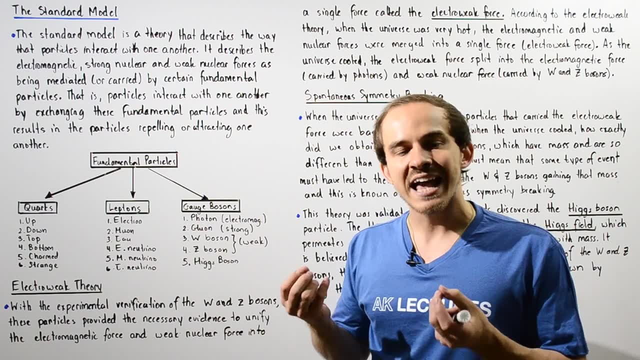 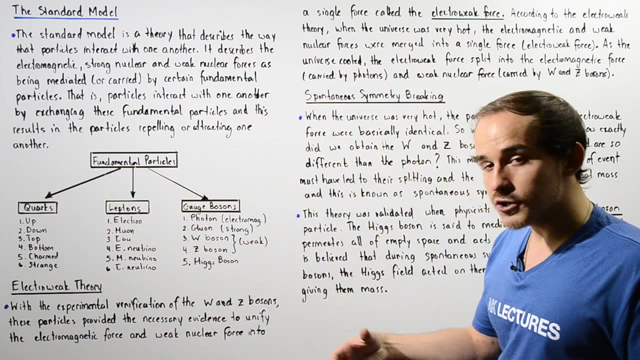 the W boson and the Z boson were basically particles that were very, very similar, if not identical, And these particles all carried the same exact force, known as the electroweak force. Now, as the universe cooled, what happened was the electroweak force. 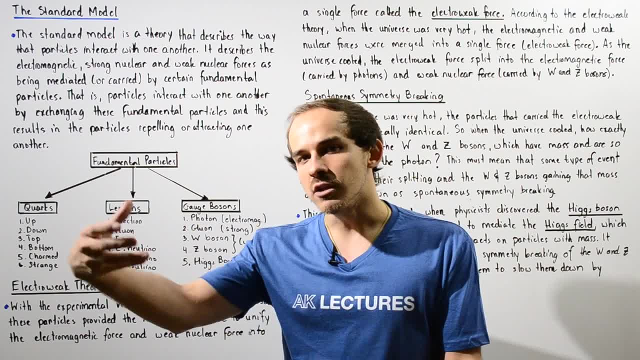 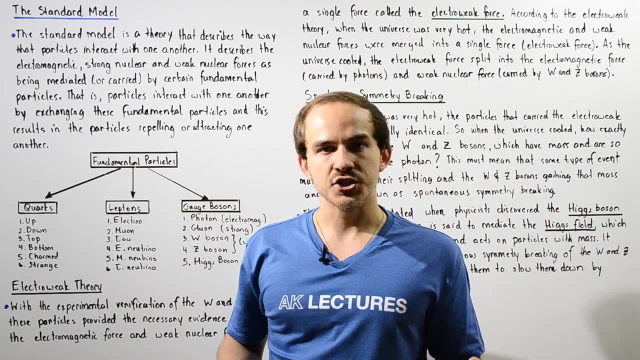 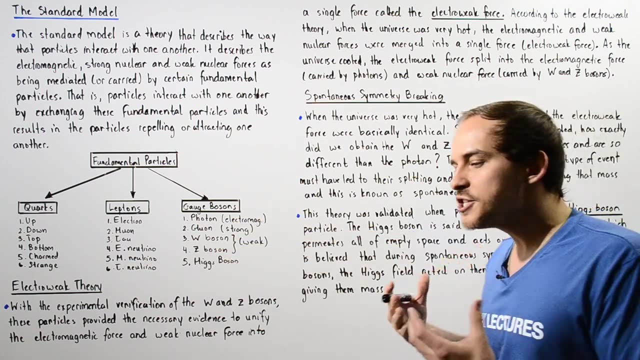 splintered. The electroweak force splintered into two different forces: the electromagnetic force, which was now carried by the photon, and the nuclear force, the weak nuclear force, which was now carried by the WNZ boson. Now, when the splitting took place, our WNZ bosons gained. 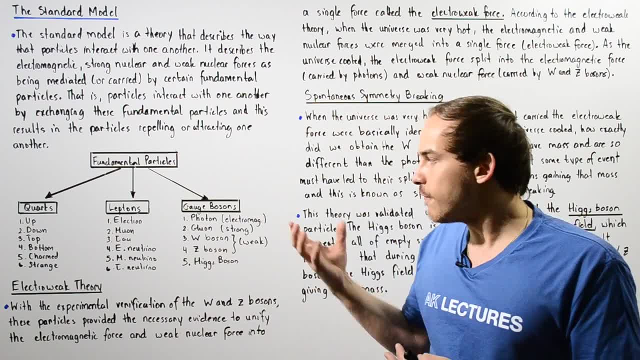 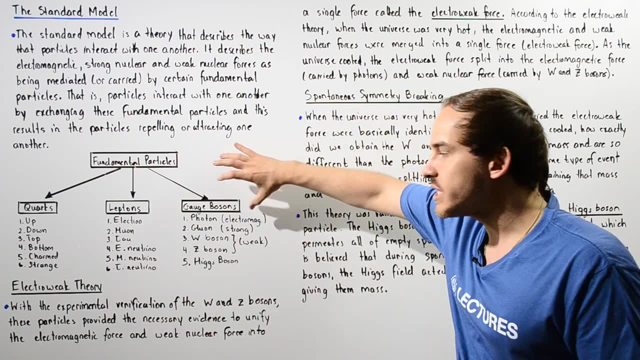 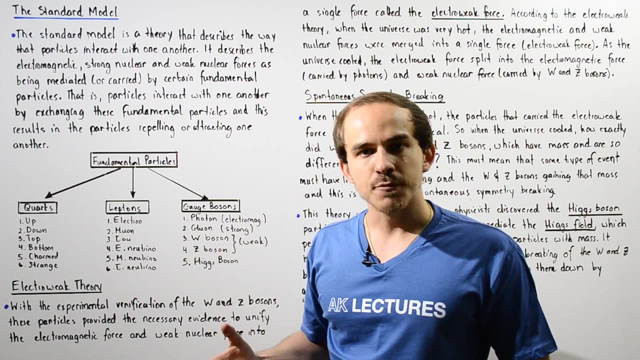 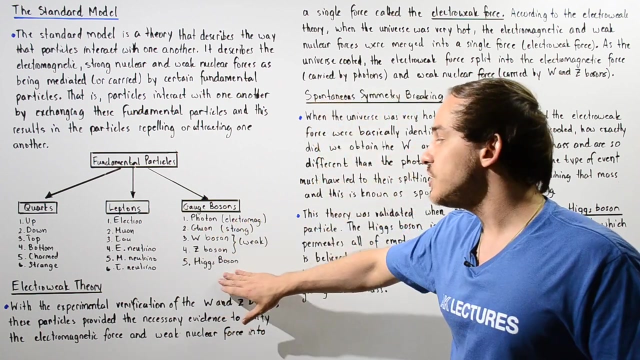 a lot of mass. So before the splitting the photon the WNZ bosons were very similar. But after our splitting, the photon basically remained massless but the WNZ boson gained a lot of mass. And the way that we explain how this mass was gained by the WNZ boson is by using the 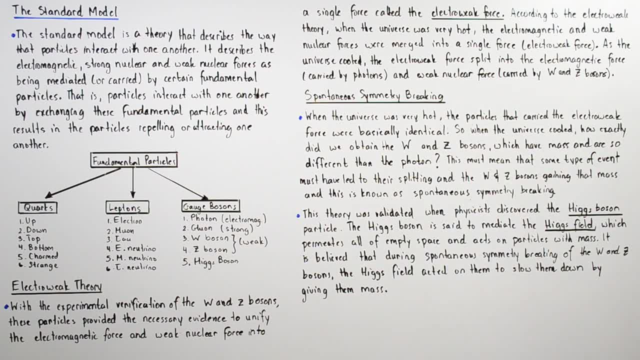 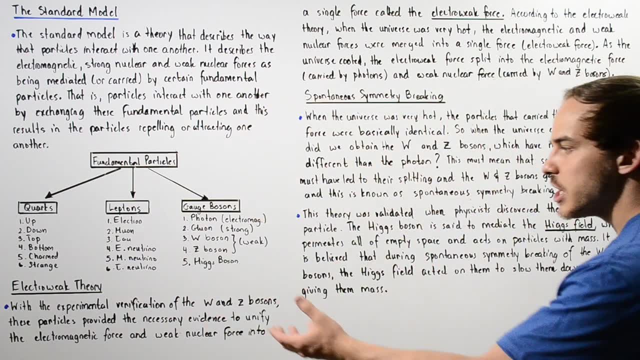 Higgs boson particle, as we'll see in just a moment. So, once again, with experimental verification of the WNZ bosons, these particles probably gained a lot of mass, And the way that we explain how this mass gained this mass by using the Higgs boson particle, as we'll see here in a minute, are 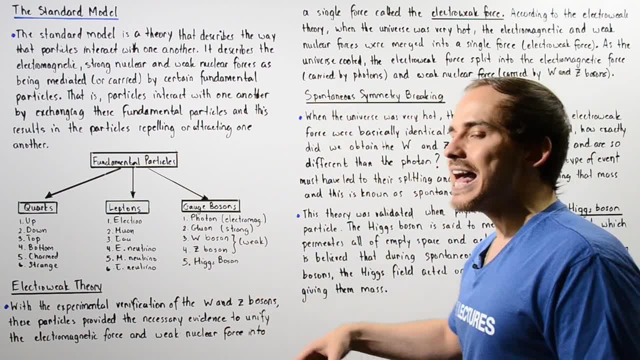 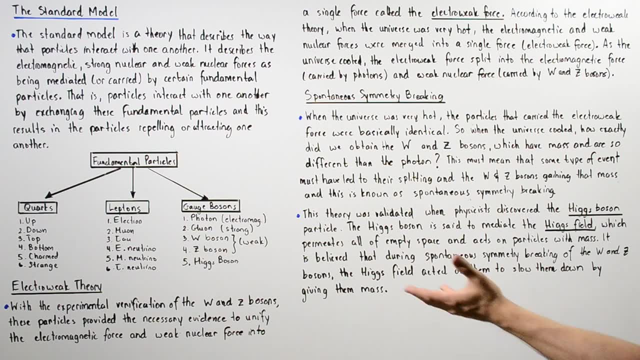 what we call the electromagnetic force. Now, with this theory, the electromagnetic force was combined with the weak nuclear force. This is the way the electron is produced: from a weak nuclear force. So the electromagnetic force was combined with a weak nuclear force. 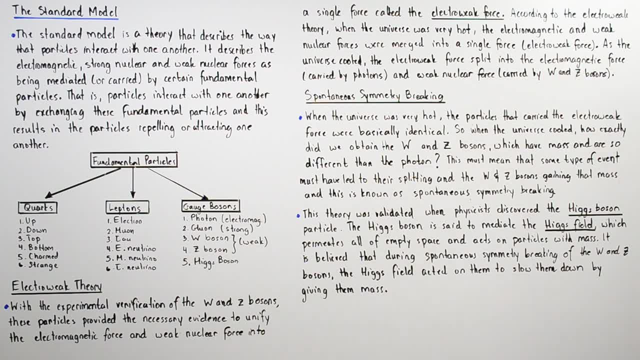 When the universe was very hot, the electromagnetic and the weak nuclear forces were combined into a single force known as the electroweak force. However, as the universe cooled, the electroweak force basically split into the electromagnetic force, which was now carried by photons, and the weak nuclear force. 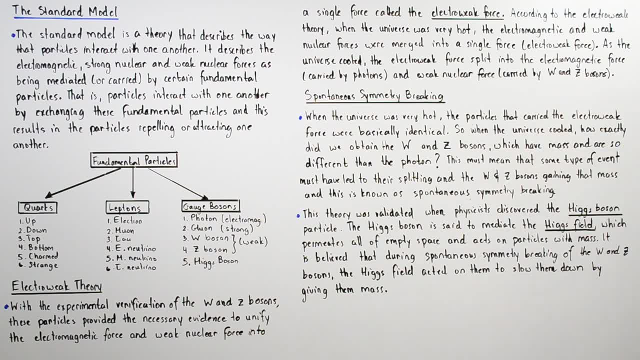 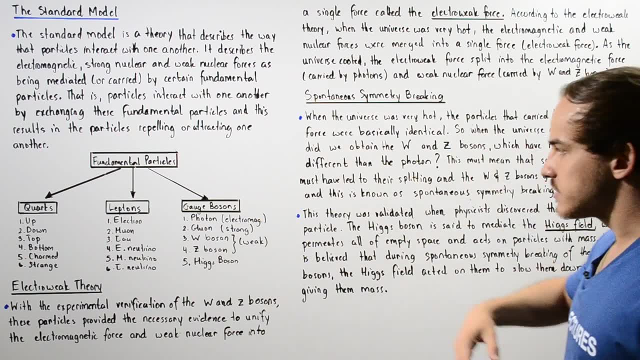 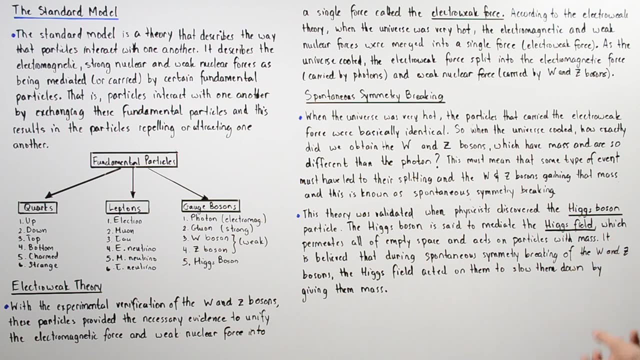 which was now carried by the W and Z bosons. Now, when the universe was very hot, as I mentioned earlier the particles, the photon, W and Z bosons. these particles basically carried one force we call the electroweak force, and these particles were essentially identical, they were very similar. 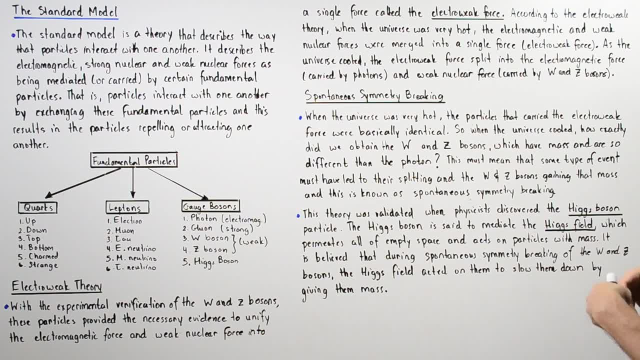 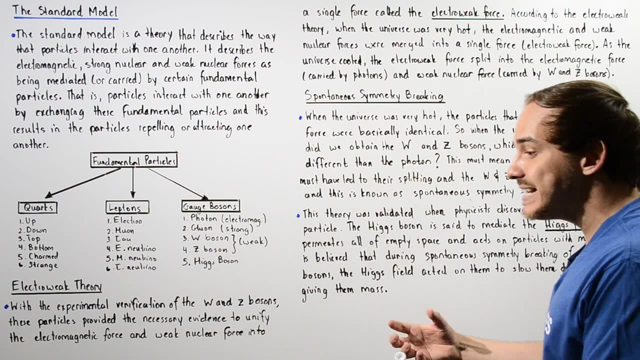 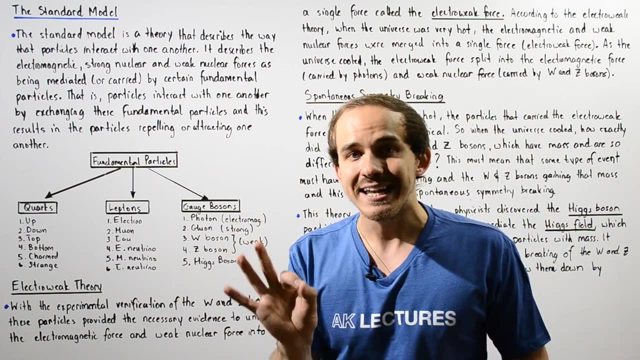 however, when the universe actually are cooled, we had the splitting take place and somehow the W and Z bosons gained this great quantity of mass. So the mass of the W and Z bosons is about 80 times the mass of the proton, and the photon, as we know, is based on the W and Z bosons. 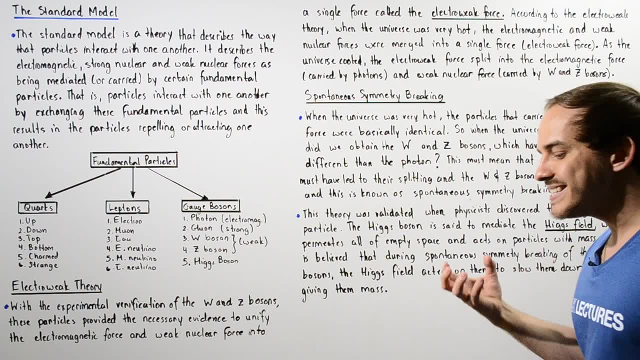 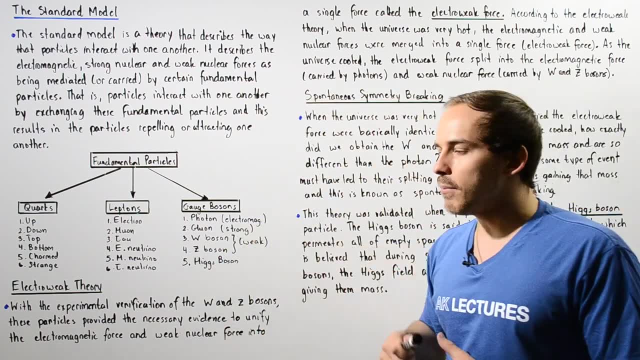 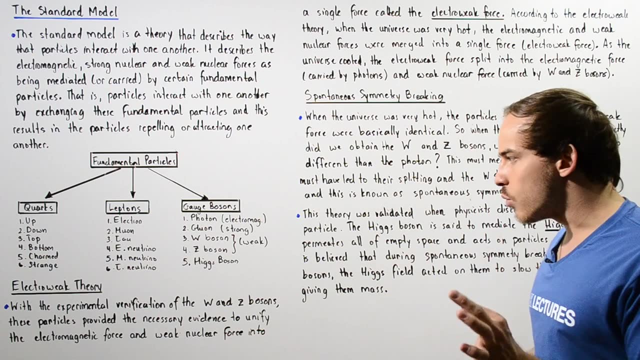 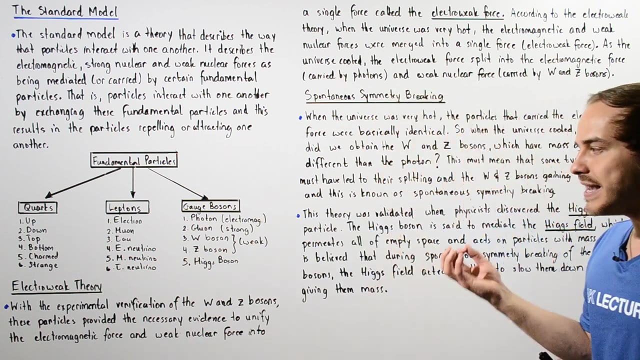 Basically massless. the question is: what exactly happened? what event took place that caused these two bosons- the W and Z bosons- to actually gain this great quantity of mass? So in 2012, the Higgs boson particle was basically confirmed experimentally, and this basically helped us. 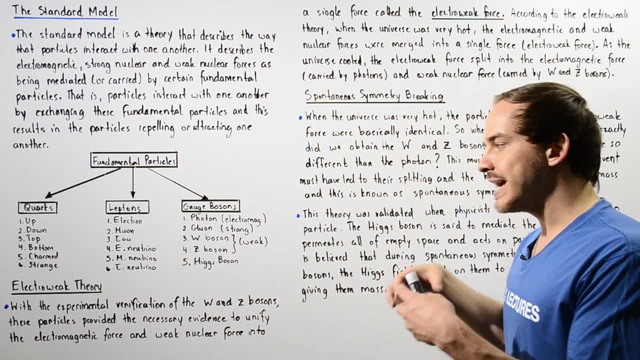 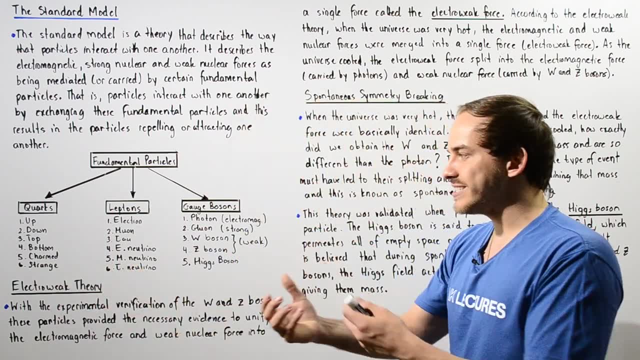 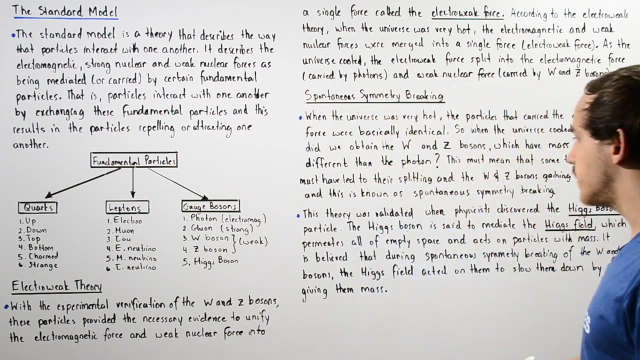 validate the electroweak theory. It helped us unify this electromagnetic force and our weak nuclear force into a single force, known as the electroweak force. that existed when the universe was very, very hot. So this theory, the electroweak theory, was validated when the physicists discovered the Higgs boson particle in 2012.. The Higgs boson 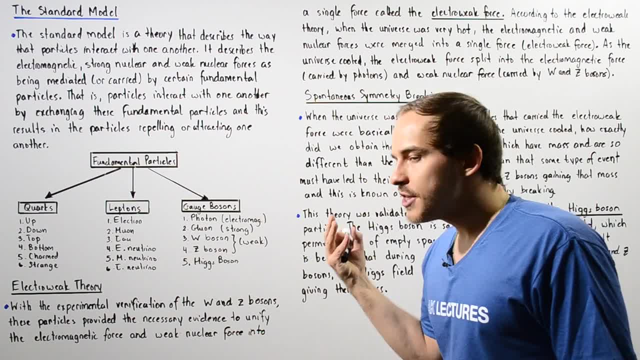 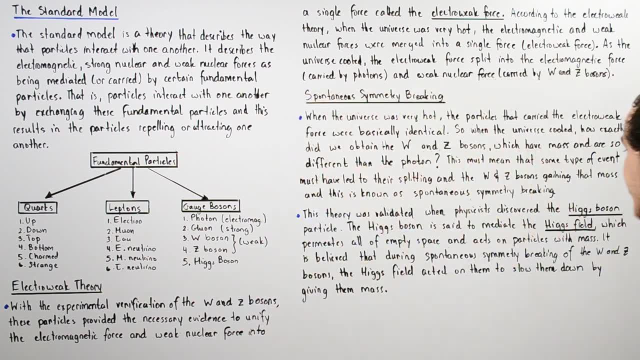 is said to carry or mediate the Higgs boson particle. When we look at the Higgs boson particle, the Higgs boson particle is essentially like a neutron. It's basically like a neutron, The Higgs boson particle, the Higgs field, and this Higgs field basically acts on any particle that has mass. Now this: 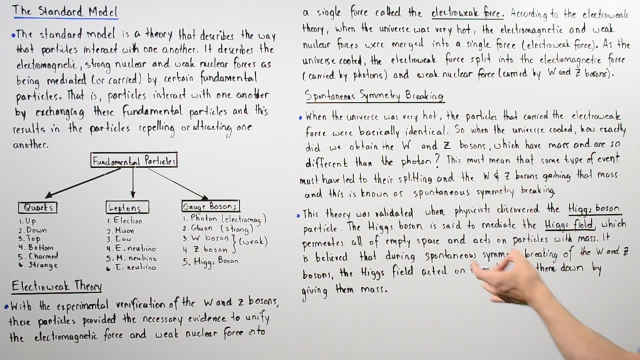 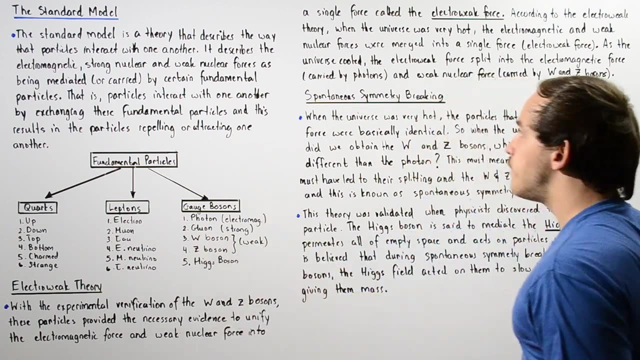 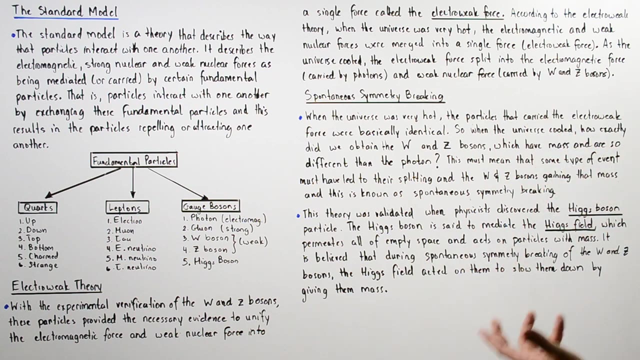 Higgs field was basically believed to cause spontaneous symmetry breaking. Spontaneous symmetry breaking is the event that basically led to the splitting of our W and Z boson and our photon, to split our electroweak force into the electromagnetic force and the weak nuclear force. 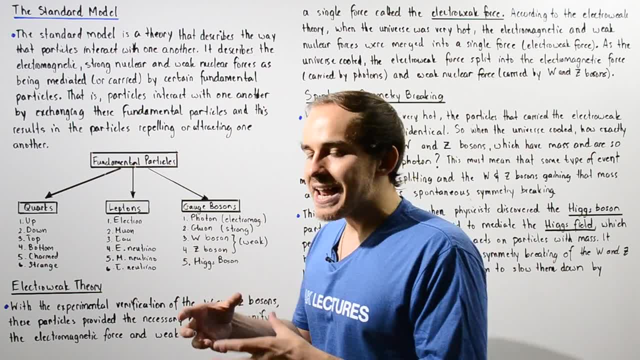 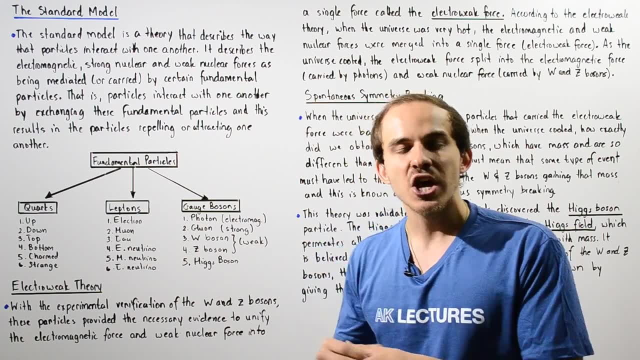 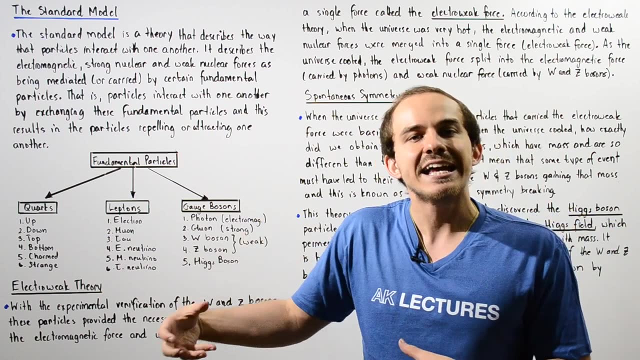 So what the Higgs field did is it acted on the W and Z bosons, which had a very, very small amount of mass, and it slowed them down, and as it slowed the velocity of these two particles, they gained mass as a result. and that's exactly what gave the W